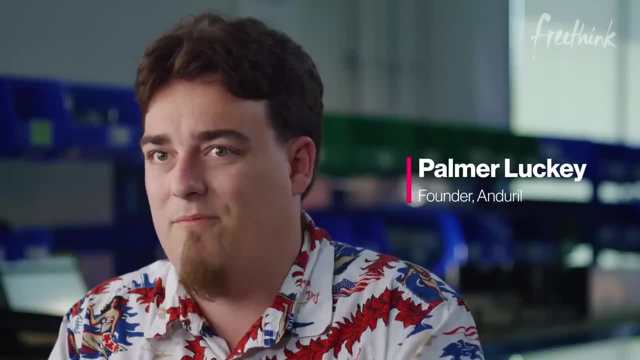 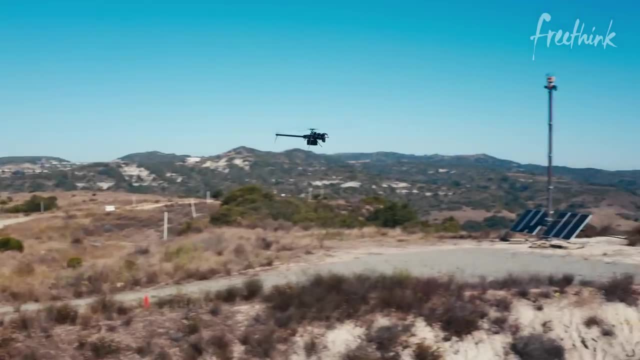 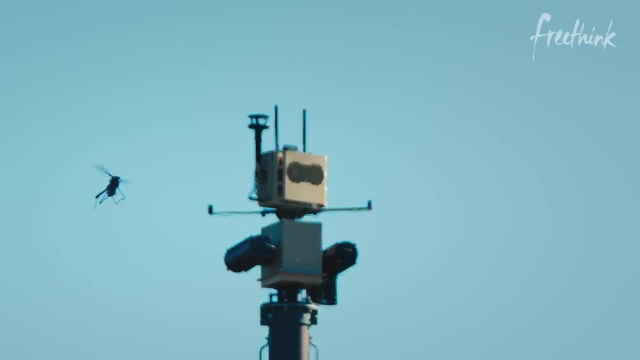 world That's starting to change. We have strategic adversaries who are rapidly surpassing us or have already surpassed us in a lot of areas. That's where our company comes in. At Anduril, we build the things that the government does not yet believe are possible. We want to build a defense product company with the. 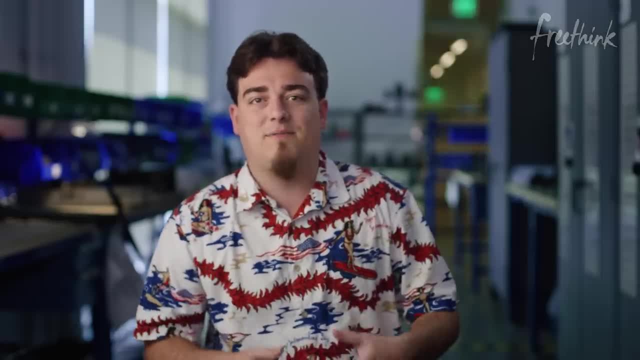 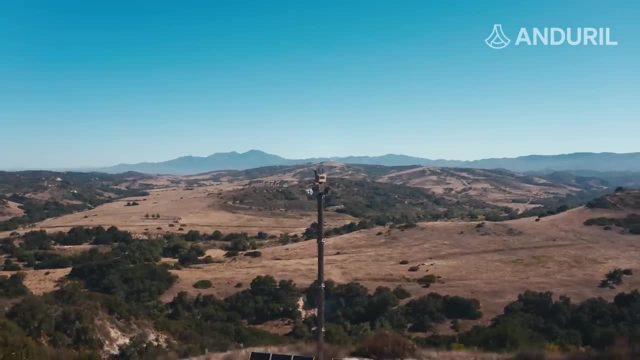 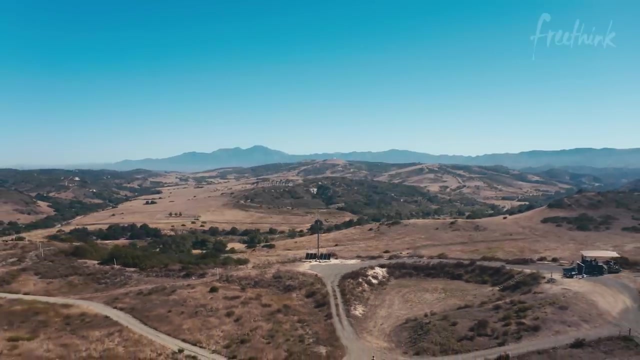 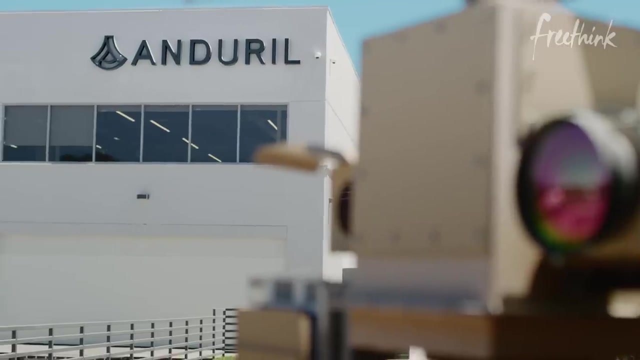 best people from the technology industry working on defense problems in the right way so that we can get things out there very quickly at very low cost and actually make an impact this year rather than ten years from now. What we're trying to do is provide warfighters with very recent, very 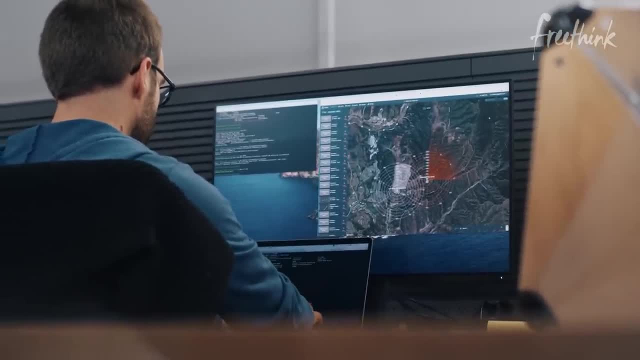 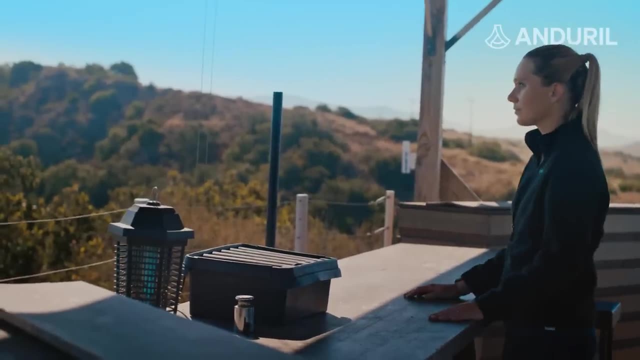 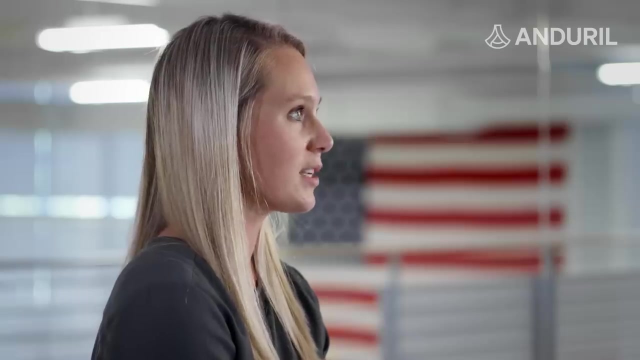 actionable, very reliable intelligence about everything that is going on around the world, Because when you have better information, you will always make better decisions. I got back from Afghanistan last year. During that time I was flying Blackhawks, piloting managing teams. You never want to be in a position where you 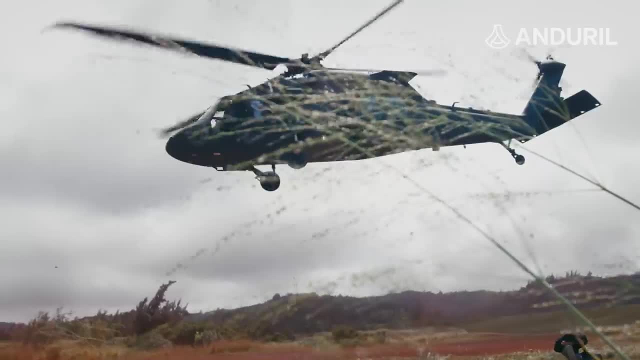 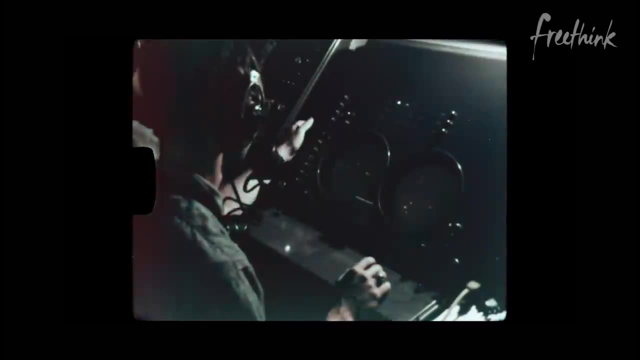 have to make a decision and you just don't have the knowledge available to you. It is something that is very near and dear to me. to make sure that our products are things that are actually creating good in the world, The world would be a very 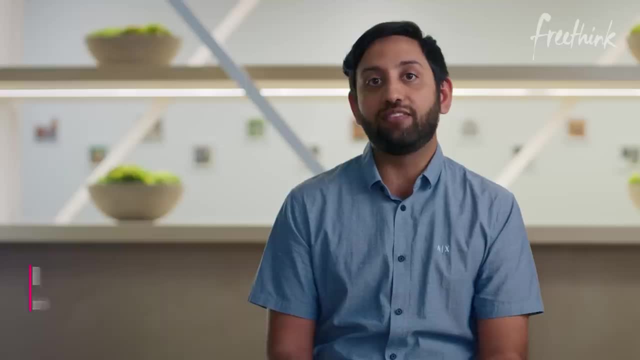 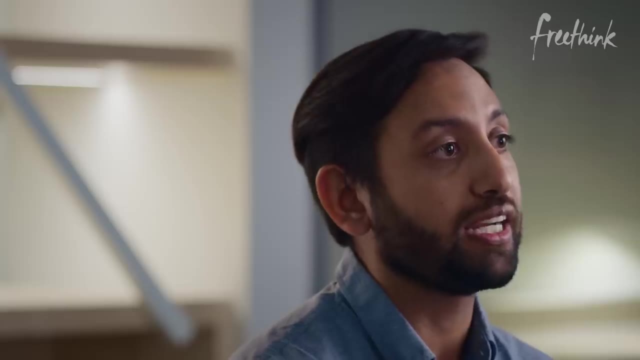 different place if In the 60s we didn't have the level of focus and effort behind developing technology solutions to protect our allies. What's a little disheartening is in modern times, the best and the brightest are not working on these kinds of problems. 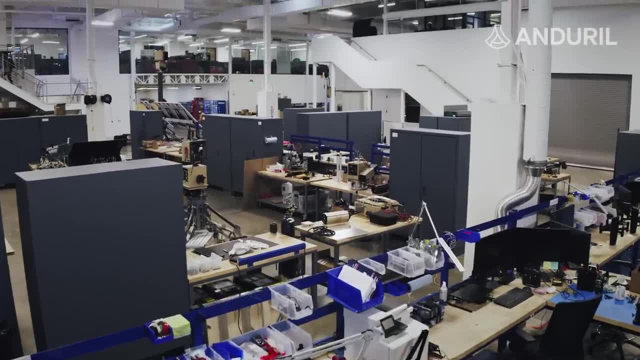 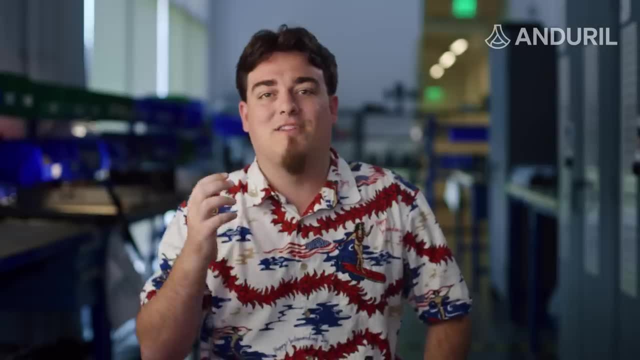 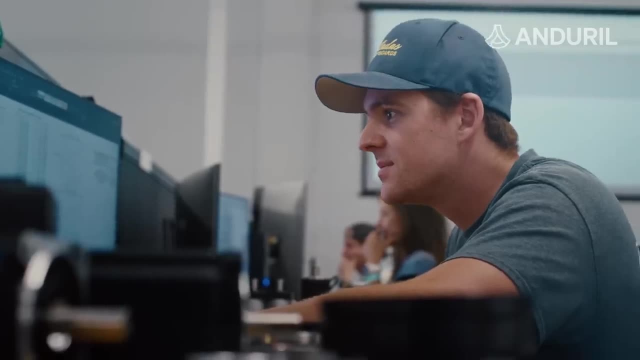 They're working on ads. So what we have here is an integrated facility where there is everything that we need to go from napkin sketch to a fully developed hardware and software product that is going out the door and overseas. In a lot of ways, this is kind of like an amusement park for an engineer. 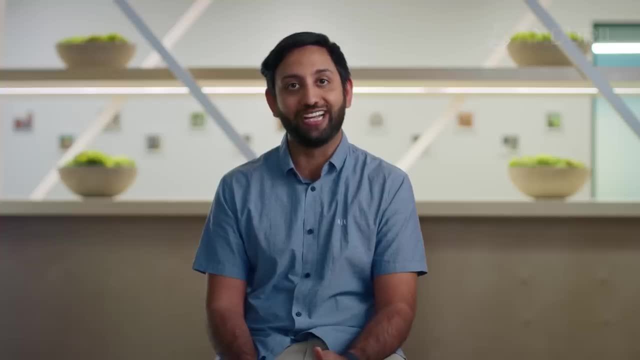 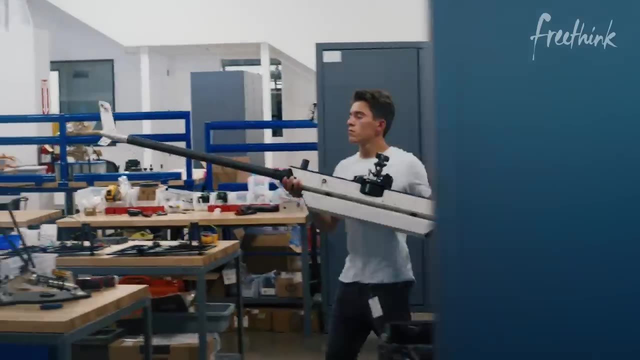 The pace at which we solve some of these problems is dizzying in some ways. So Anduril moves extremely quickly. I've been here multiple times where you see something on a Monday and it's just an idea, and then you see a prototype of it on Friday. 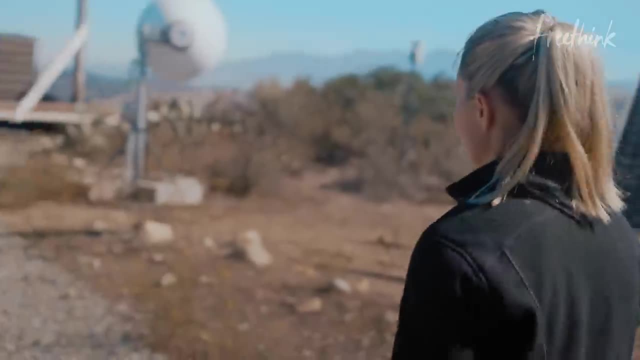 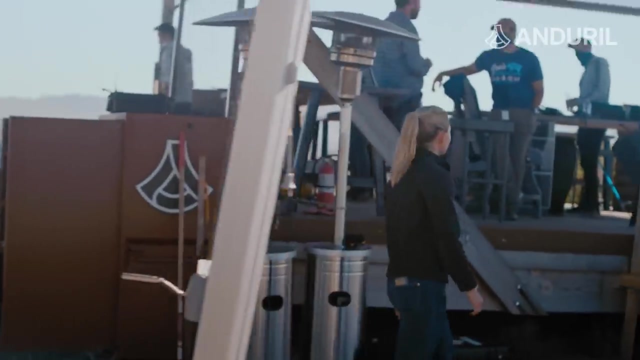 The Capistrano test site is hugely important for a company like ours. It's about 2,700 acres. We're able to test our hardware and our software in real-world conditions with our engineers. So Ghost is a battery-powered small UAS. 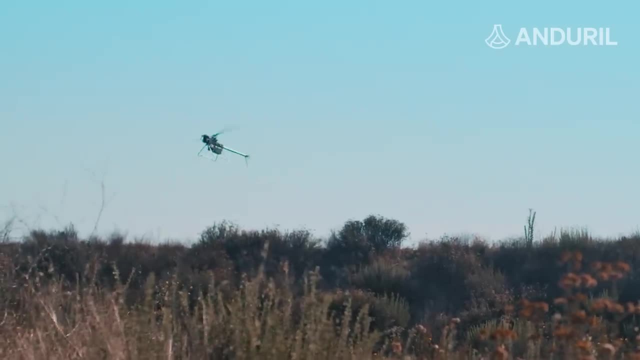 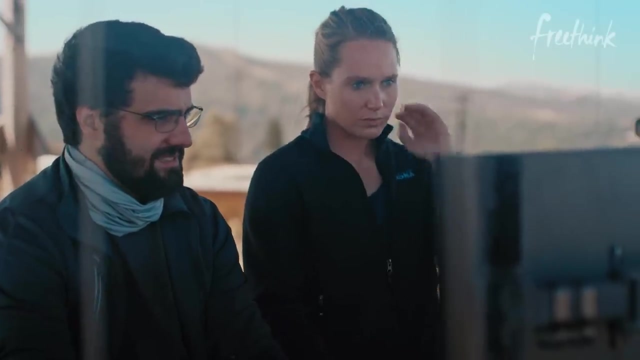 It does vertical takeoff and landing. It can fly for almost two hours virtually silent. But I don't want to get bogged down in the specifics of what the airframe does, because it's really more about Lattice and the ability to have all of your feeds interconnected. 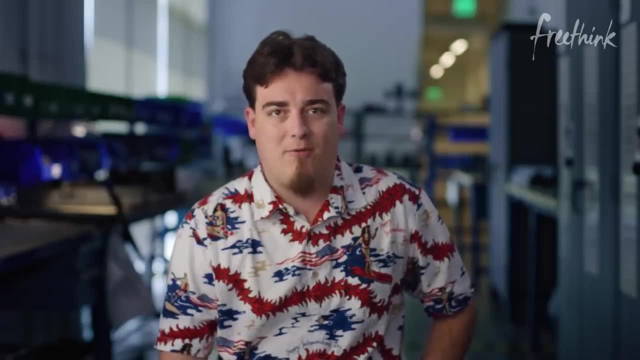 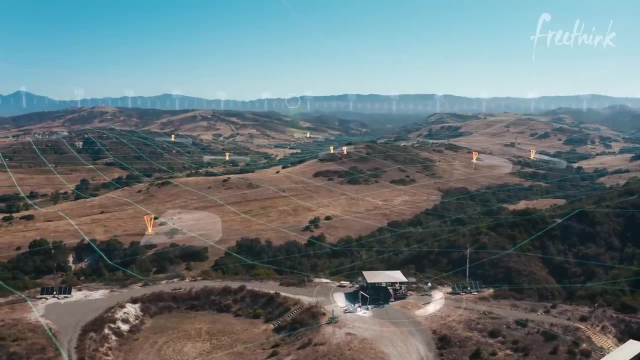 Our core product is something that we call Lattice. It's an AI-powered sensor fusion network that can take data from hundreds or thousands of different sensors across land, sea and land And it can merge them into a single common operating picture that all of the people can reference and all of the machines can reference. 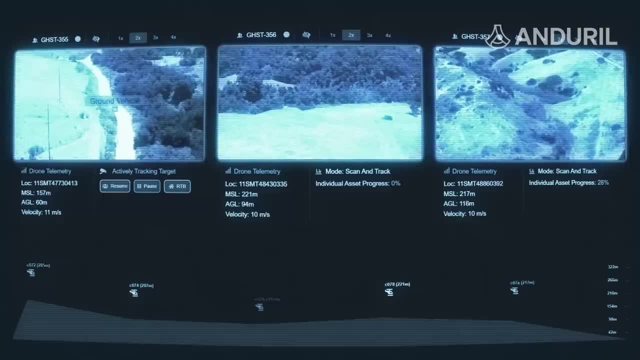 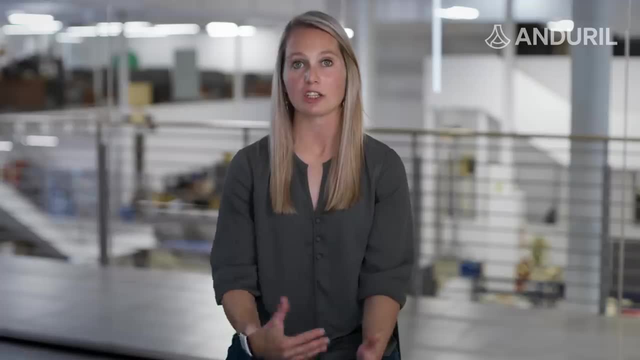 You know, showing what's going on not just now but what's going to be happening in the future. So you can have our sentry towers, you can have Ghosts all operating within the same area, and then it alerts you when there's something there that needs your action. 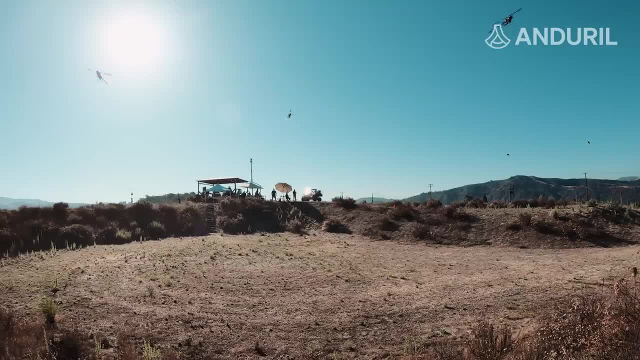 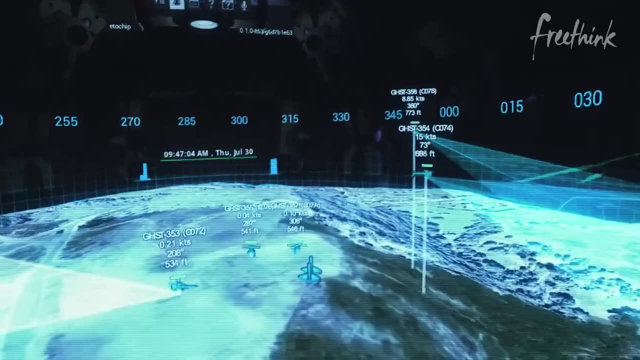 So normally you would have 10 or 15 people looking at all different screens and trying to fuse that information together. But we're able to fuse those tracks into one user interface, have one person looking at that And the ability to connect all those things. 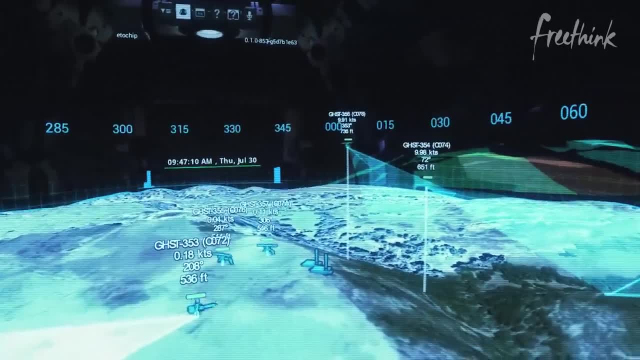 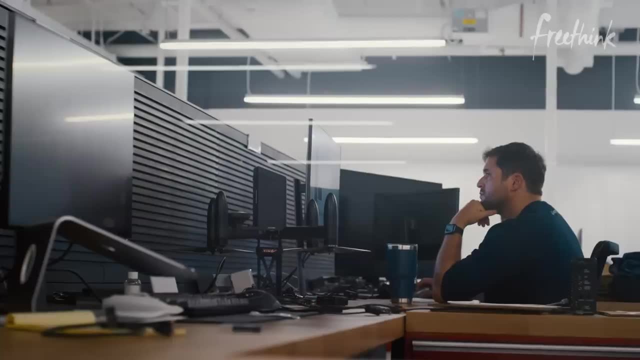 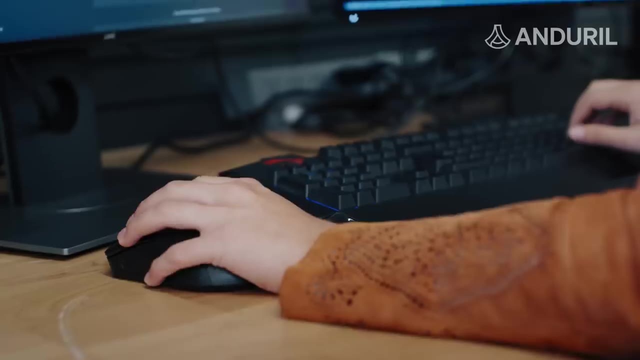 and make an operating picture to provide you better situational awareness is something that other companies are just not doing. Like every other company, we have sketches, we have ideas, we have things that we want to work on. The difference here is that we don't take those sketches. 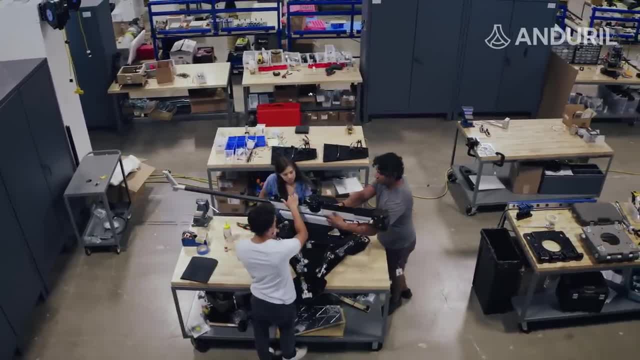 and then go to the government and ask them to help us make them, If we believe it's the right thing that needs to be done. If we believe it's the right thing that needs to be done. If we believe it's the right thing that needs to be done. 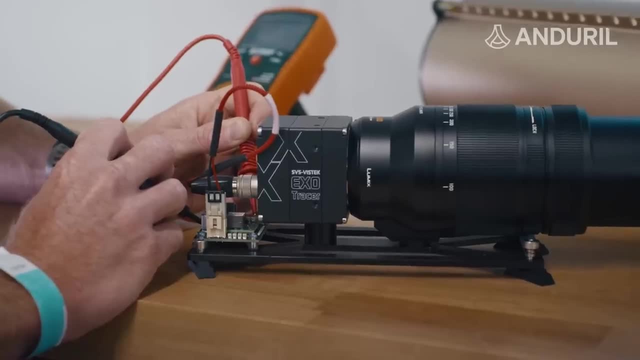 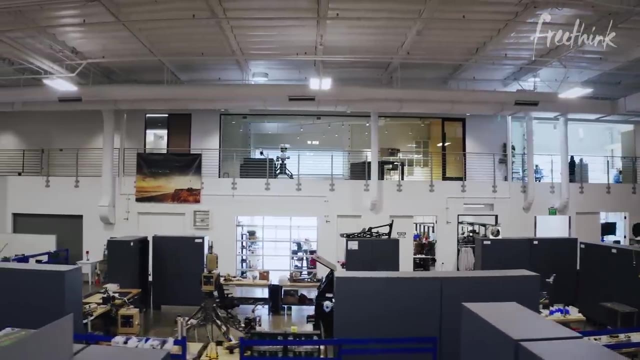 if it's the right thing that needs to exist, we're going to make it exist, regardless of whether or not people believe it's possible or are willing to give us money. That's a pretty unique thing in the defense space And I am going to make sure that we never lose that. 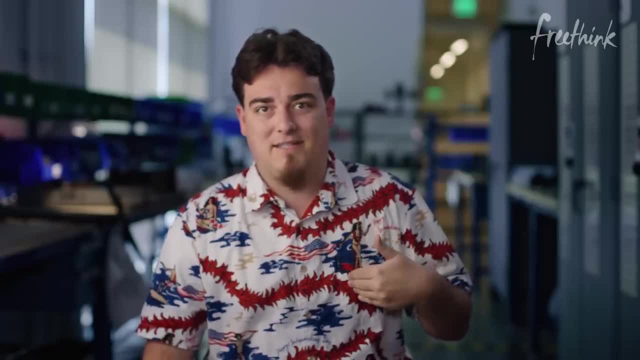 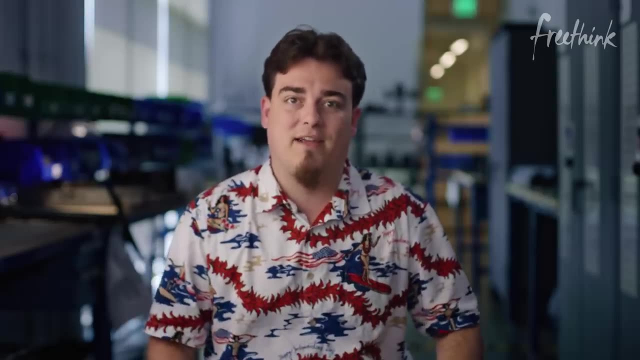 So I'm working on defense technology because I believe in it, because I think it's important to work on and because not enough people are working on it, And I'm one of the people who's blessed with the resources to actually have a shot at making a difference. 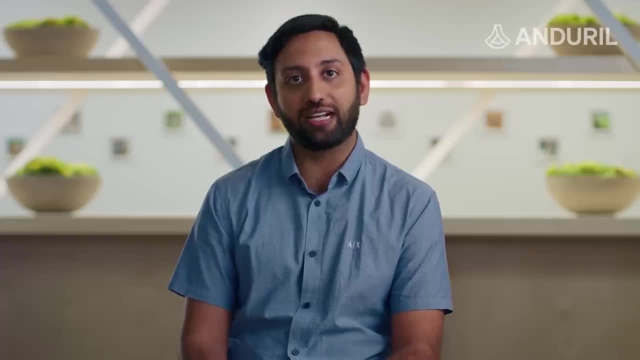 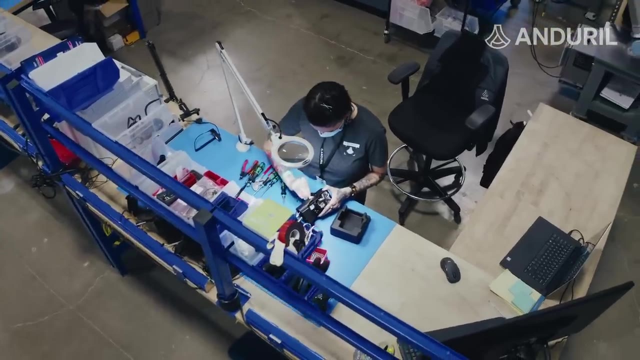 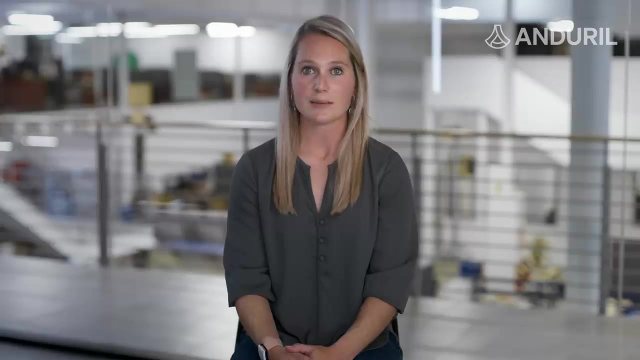 I could see the impact of the problems I was working on directly. where you're protecting our nation's security, keeping our bases safe. I think Anduril has the potential to make incredible impact in the world. I've been deployed multiple times just being able to see that sometimes you're not able